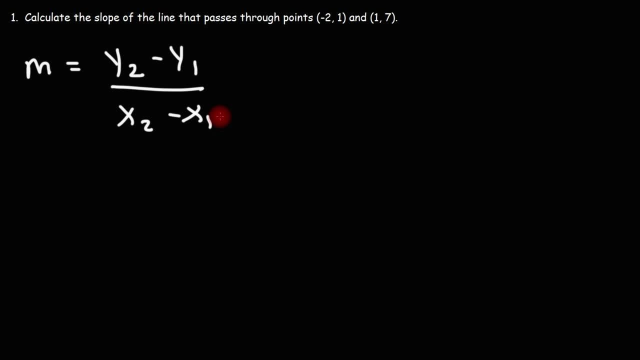 Now what you need to do is identify your x and y values in the two ordered pairs that you're given here. x is first, y is second, And let's choose a smaller font, So this is going to be x2 and then y2.. 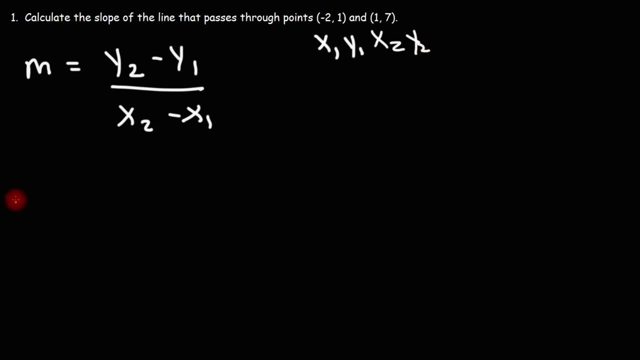 So x is the first coordinate, y is the second one. Now it really doesn't matter the order in which you write it. the answer will still be the same. So, the way we've defined it, y2 is 7,. y1 is 1,. 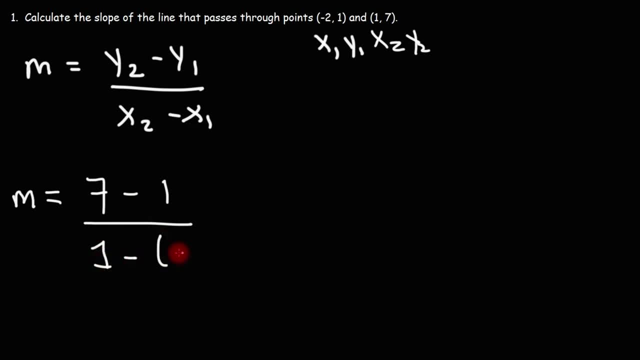 x2 is 1, and then minus x1 is negative 2.. So we have 7 minus 1, which is 6, and then 1 minus negative 2, that's the same as 1 plus 2.. A negative times a negative is a positive. 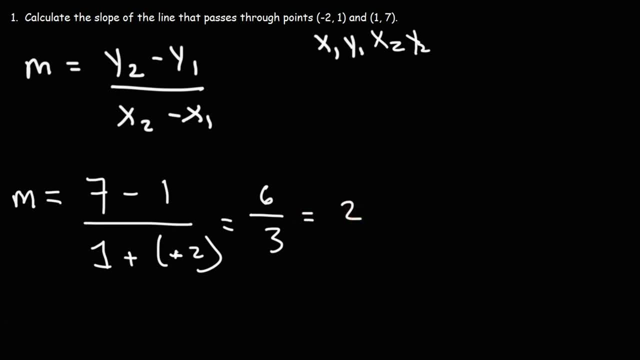 1 plus 2 is 3, so we get 6 divided by 3, which is 2.. So that is the slope of the line that passes through these two points. Another common problem that you're going to encounter in algebra is solving linear equations. Some equations might be simple, others might contain lots of variables. 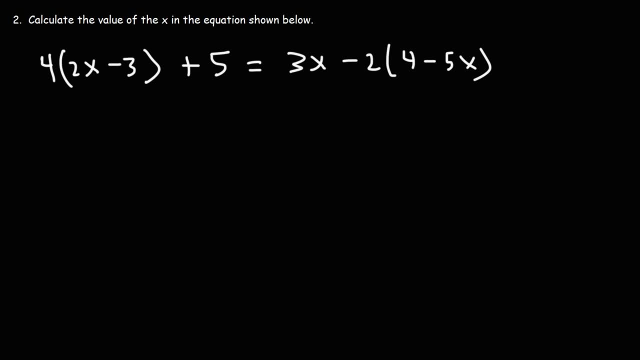 and parentheses, and sometimes even decimals and fractions, But let's work on solving this one. The first thing we need to do is distribute. Let's distribute 4 to 2x minus 3.. 4 times 2x is 8x. 4 times negative 3 is negative 12.. 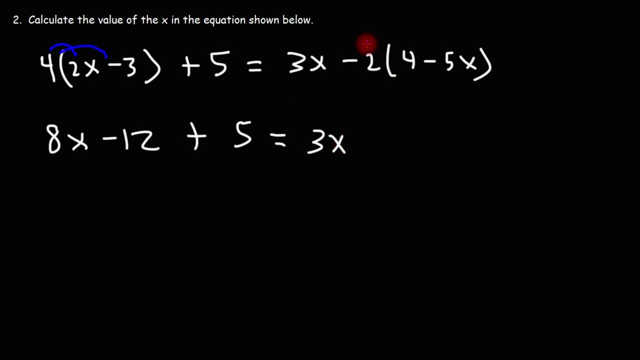 Now let's do the same thing on the other side. Let's distribute negative 2 to 4 minus 5x. Negative 2 times 4 is negative 8, and then negative 2 times negative 5x, that's going to be positive 10x. Now the next thing we need to do is we need to add like terms: 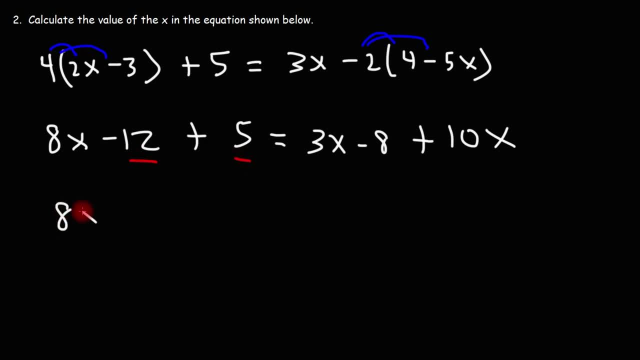 So we can add negative 12 plus 5, that's going to give us negative 7, and we can also add 3x and 10x- that's going to give us 13x. Now we need to get x by itself on one side of the equation if we want to calculate its value. 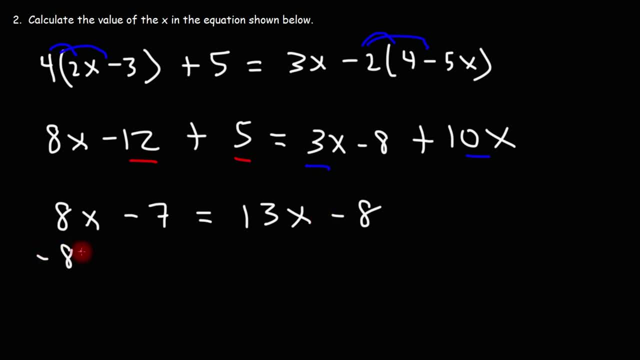 To do that, let's subtract both sides by 8x and let's add 8 to both sides. This will put all of the x variables on one side of the equation and all of the non-x variables on the other side. Negative: 7 plus 8 is 1,. 13x minus 8x is 5x. 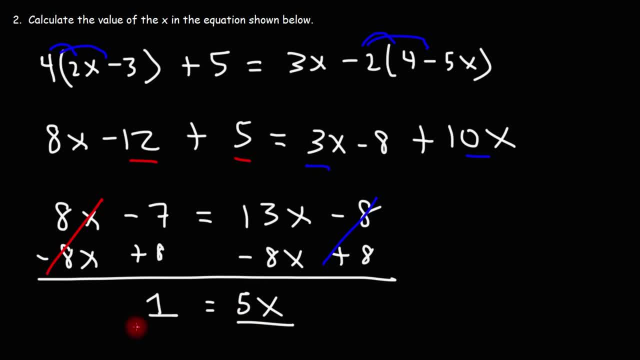 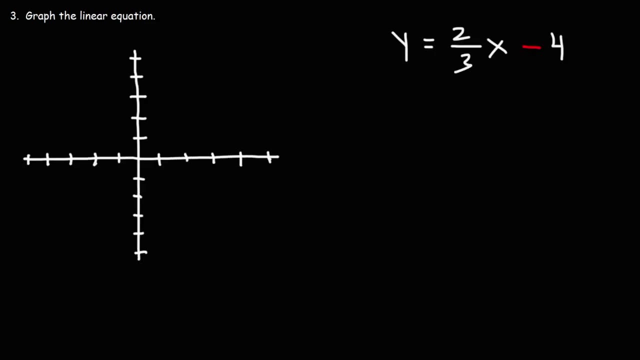 so we get: 1 is equal to 5x. Now to get x by itself, We got to divide both sides by five. So the answer is one over five. That's the value of x. The next typical problem that you'll face in algebra is graphing linear equations. 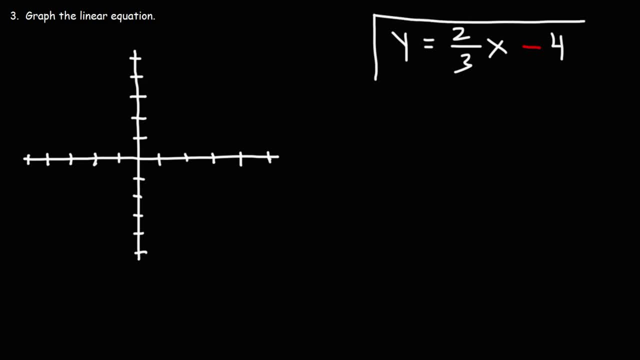 So here we have a linear equation in slope and in step form, y equal two over three, x minus four, And we need to graph it. So how can we do that? Well, first you need to realize that this is in: y equals mx plus b, format slope and in step form, m is the slope, m is the number in. 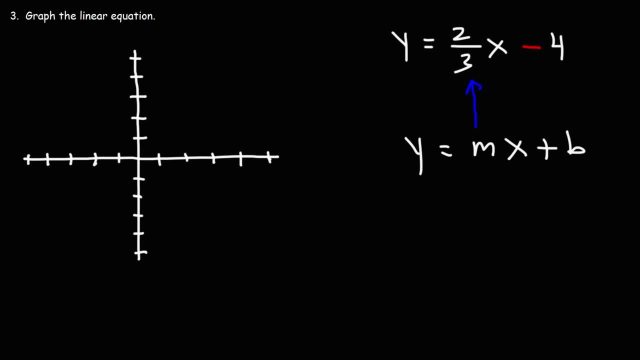 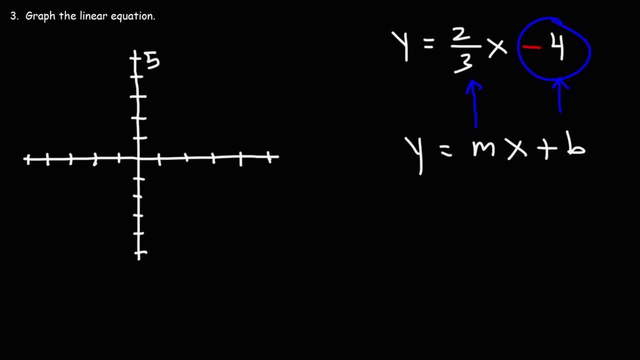 Negative four, And this is where the line touches the y-axis. So negative four is right here, along the y-axis. This is the y-axis, This is the x-axis. Now, in order to graph a linear equation, we only need two points. We already have the first point, the y-intercept. 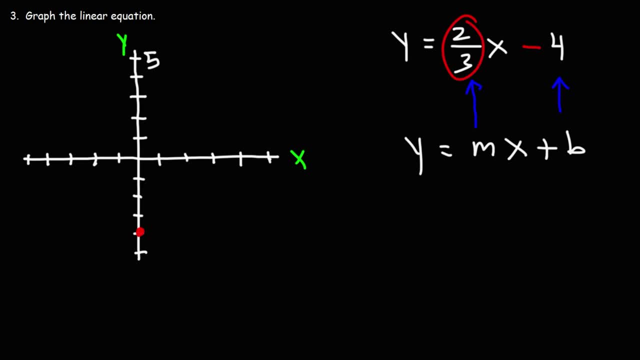 We can use the slope to go from the first point to the second point. So the slope is two over three. The slope is equal to rise over run. So to get the next point, we're going to rise two units and then run three units to the right. So we're going to go up two. 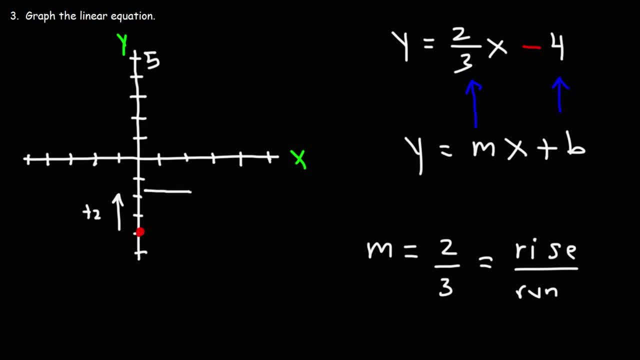 and then over three. So the next point: it's going to have a y-value of negative two, but an x is value of three. Now we just need to connect the two points with a straight line And that will give us the answer. So that's how we can graph a linear equation in slope intercept form. 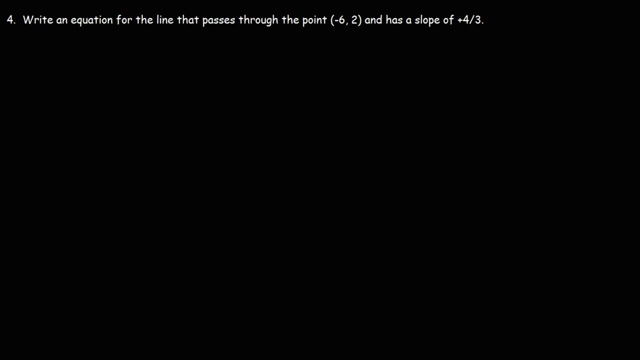 Now the fourth type of question that you're going to see in a typical algebra course has to do with write-in linear equations, And there's many variations of this type of question. You could be asked to write a linear equation of a line that passes through a point. 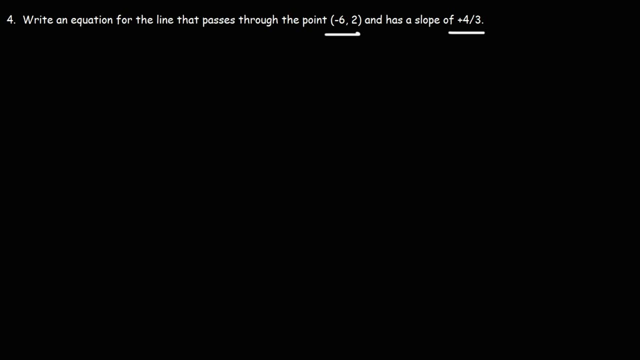 and you're given a slope. Sometimes the line you're given the two points that the line passes through, Other times you're given one point and the equation of a line parallel to the line that you want to write an equation for. Other times they'll give you a line that's perpendicular. 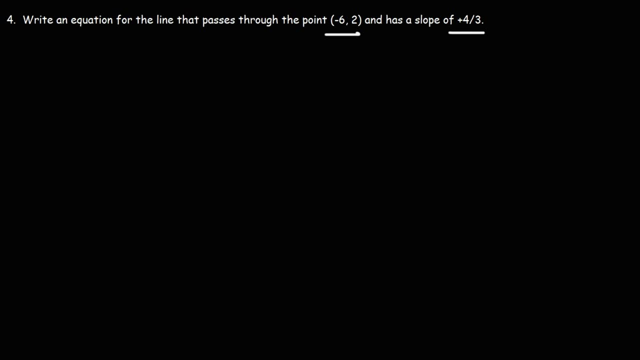 to the line that you want to write an equation for. So you're going to have one of those variants of this kind of question. Now, one thing I didn't specify with this type of problem is what form we should write. the linear equation in The most common form is slope intercept form. y equals mx plus b. So if it's 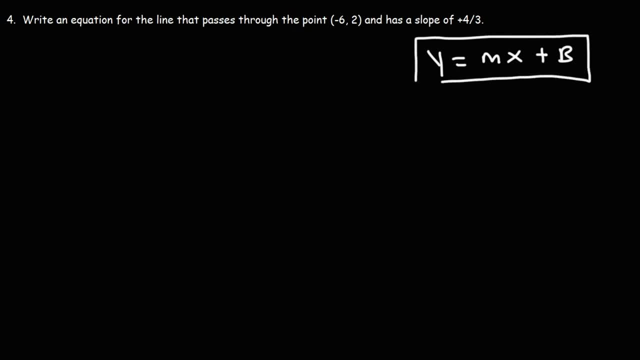 not specified. this is the default way to write the equation. If the problem says to write it in standard form, you want to put it in ax plus by equals c format. If it asks to write the equation in point-slope form, then you want to put it in this format. So those are the three common ways in which you can. 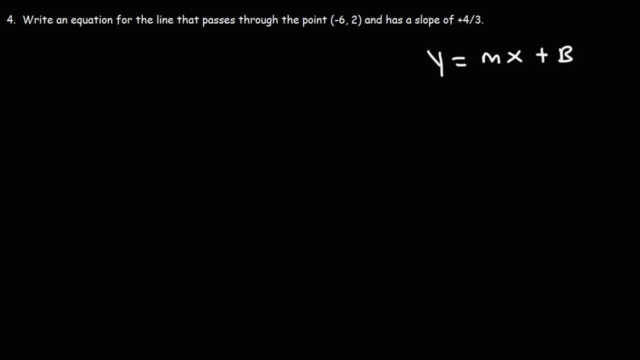 write a linear equation. We're going to focus on the slope intercept form of the equation, Since we already know the slope: it's 4 over 3.. All we need to do in this problem is calculate the value of b, the y-intercept. Now we have the value of x and we know the value of y. 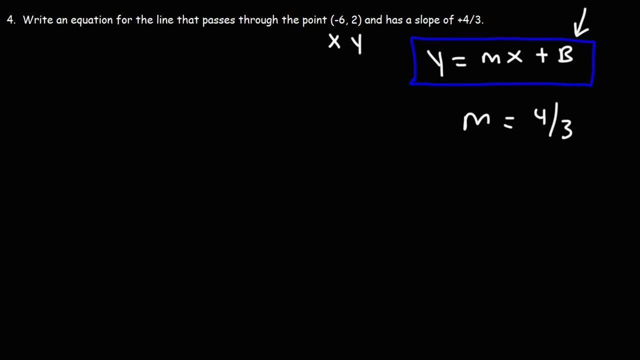 and we have m. If we plug in those three things, we can calculate b. So y is 2, m is 4 over 3, x is negative 6, and now let's find b 4 times negative. 6 is negative 24 divided by 3.. Negative 24 divided by 3 is negative 8.. 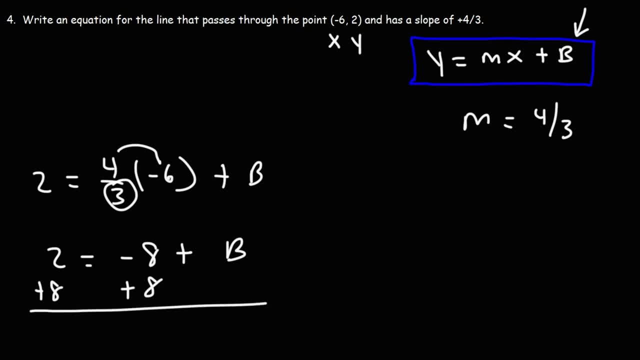 To get b we need to add 8 to both sides. So we have b by itself on the right side. On the left we have 2.. We have 2 plus 8, which is 10.. So b is 10. When you know the y-intercept and the slope. 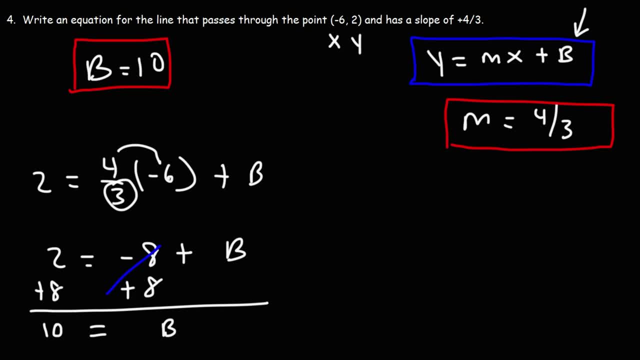 you have everything that you need to write the linear equation. So let's go ahead and replace m and b in this equation, So it's y is equal to 4 over 3x plus 10.. So that's how we can write the linear equation. if we're given the slope and a point that the 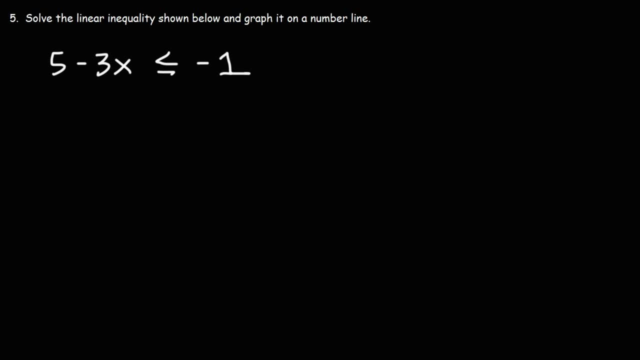 line passes through. The next common topic has to do with linear equalities. So how can we solve this linear equality and how can we graph it on a number line? Sometimes you may be given linear equalities with absolute value equations, So that's another common topic in algebra. But let's focus on solving this linear equality. 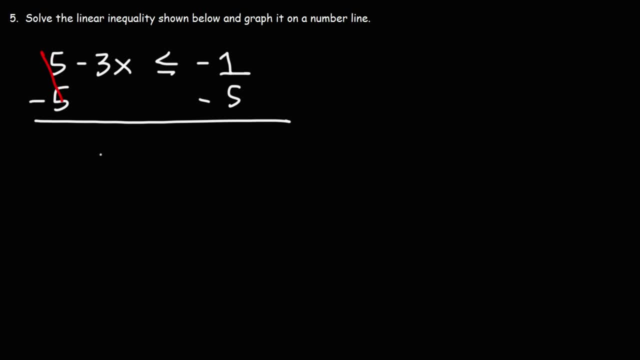 Let's subtract both sides by 5.. We'll cancel the 5 on the left side. on the right side, we have negative 1 minus 5, which is negative 6.. Now we need to get x by itself. So let's divide both sides by negative 3.. 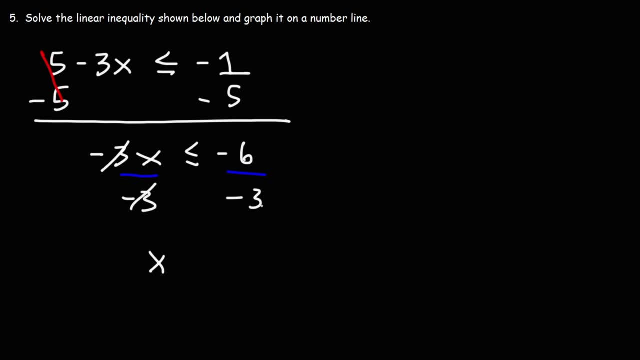 Now, when dealing with inequalities, whenever you multiply or divide both sides by a negative number, the direction of the inequality changes. So we have negative 6 divided by negative 3, which is positive 2.. So the answer is that x is equal to or greater than 2.. 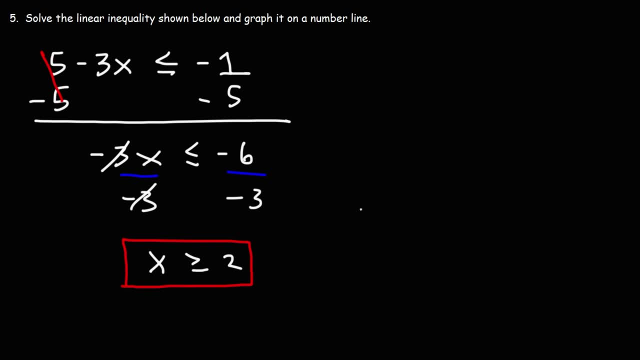 Now let's go ahead and plot that solution on a number line. So here's 0.. 2 is to the right of that. Now this is greater than, or equal to, 2.. So then we're going to have a closed circle instead of an open circle, And because it's greater than 2, we're going to shade to the right. 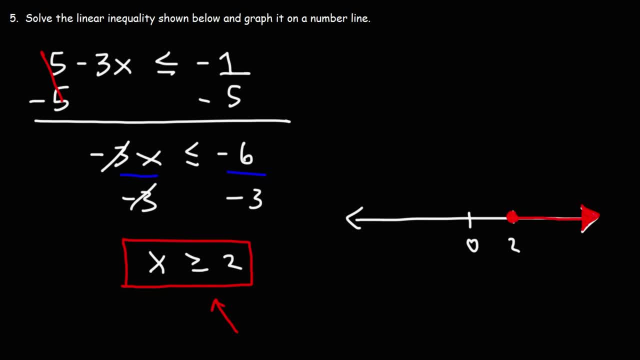 So that's how you can show your solution on a number line. Now the next most common type of problem is when you have a number line that's greater than or equal to 2.. Now the next most common type of problem you're going to see in a typical algebra course. 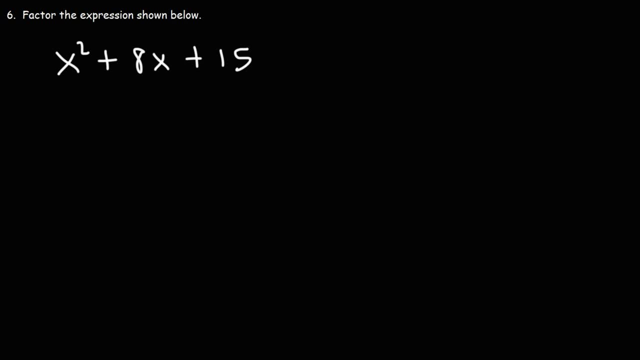 is factoring, Factoring trinomials, binomials, even polynomials, In fact, a course wouldn't be an algebra course without this type of problem. So how can we factor this trinomial where the leading coefficient is a 1?? 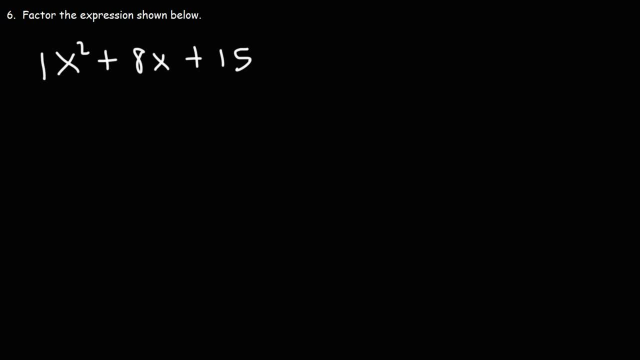 A simple trick is to find two numbers that multiply to the constant term 15, but that add to the middle coefficient 8.. And these two numbers are 5 and 3.. 5 times 3 is 15, but 5 plus 3 is 8.. 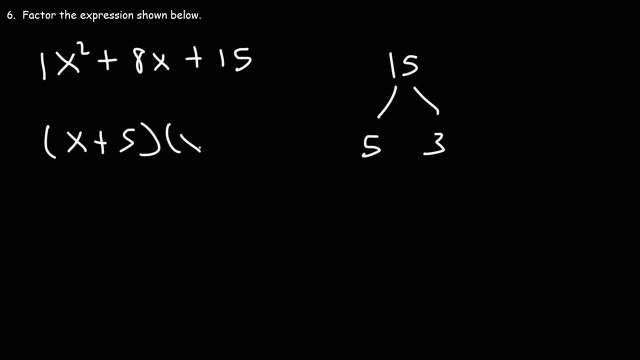 So, to factor it, it's going to be x plus 5 times x plus 3.. So that is the answer. Now, if you want to check your work, if you want to make sure you have the right answer, all you need to do is FOIL these two binomials. 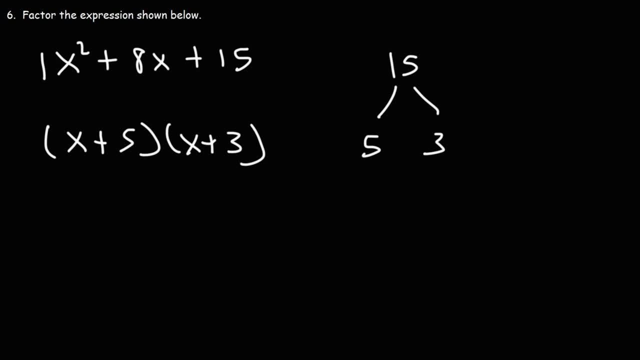 FOILing is the reverse process of factoring. When you factor, you're going in this direction, When you FOIL, you're going backwards. So let's make sure we have the right answer. x times x is x squared, x times 3 is 3x. 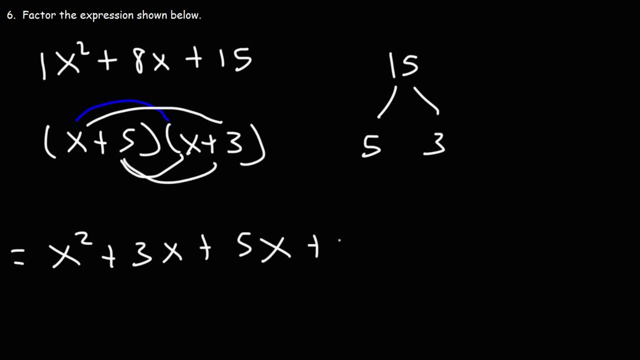 5 times x is 5x, 5 times 3 is 15.. And then we'll add the two like terms: 3x plus 5x is 8x. So it gives us the original problem. Therefore, this answer is indeed correct. 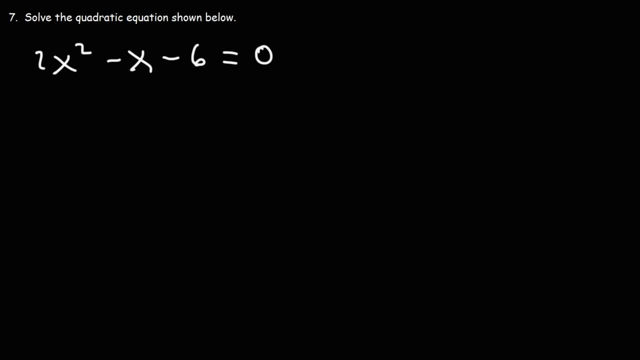 The seventh most common type of problem that you're going to see in a typical algebra course has to do with quadratic equations, particularly solving them. Now, there's a variety of methods that you can use to solve this quadratic equation. You can factor it, you could use the quadratic formula. 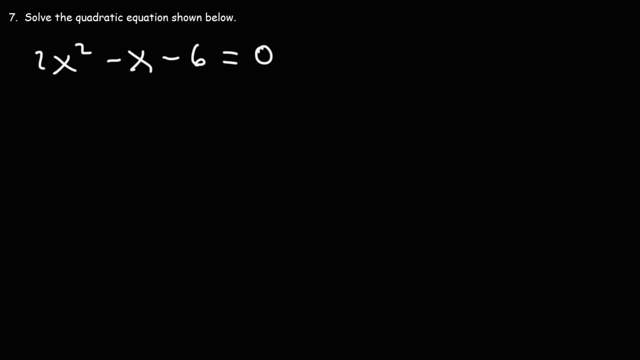 or you could use the completing the square method to get the job done. If you want to use the quadratic formula, the equation has to be in standard form, which it is, And you can see that a is 2.. b is the number in front of x. 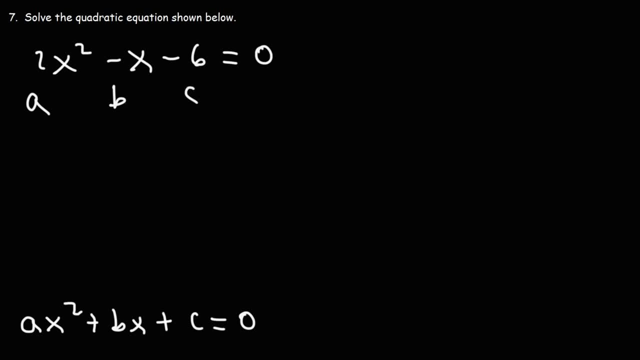 So b is negative 1.. c is negative 6.. And here's the formula: x is equal to negative b, plus or minus the square root of b squared minus 4ac divided by 2a. Now let's go ahead and plug everything in to this formula. 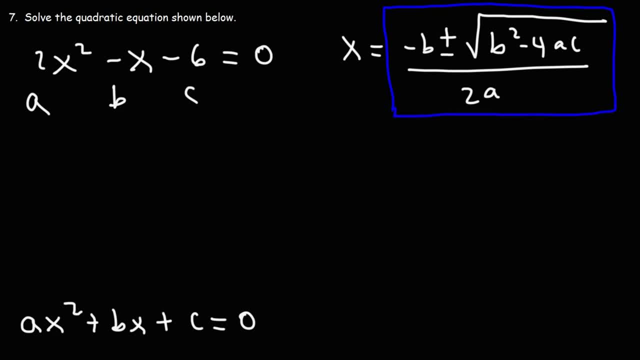 Let's get the answer. So we have negative and then b is negative 1,, plus or minus the square root. negative 1 squared minus 4, times a, a is 2, and then times c, which is negative, 6,. 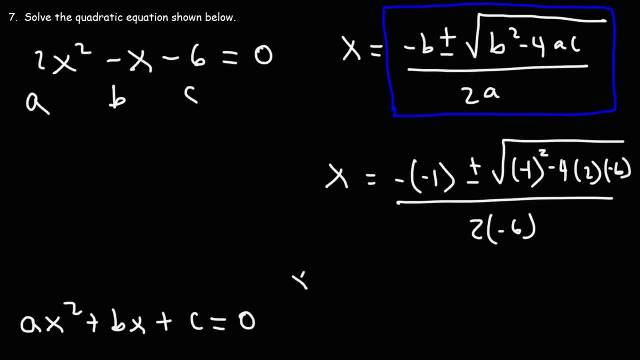 divided by 2a or 2 times negative: 6.. So negative times negative: 1 is positive: 1.. Negative 1 squared is 1.. 4 times 2 is 8.. 8 times 6 is 48.. 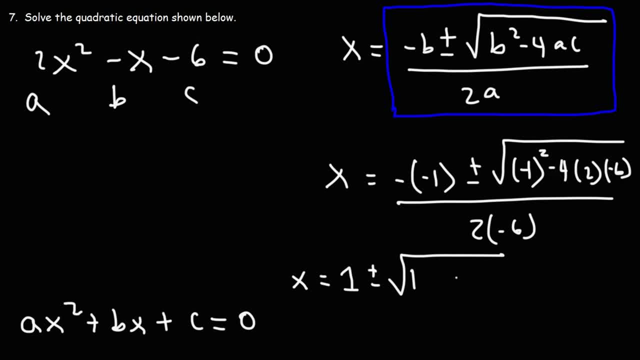 The two negative signs will cancel, giving us positive 48.. On the bottom we have 2 times negative 6,, which is negative 12.. Now 1 plus 48 is 49.. The square root of 49 is 7.. 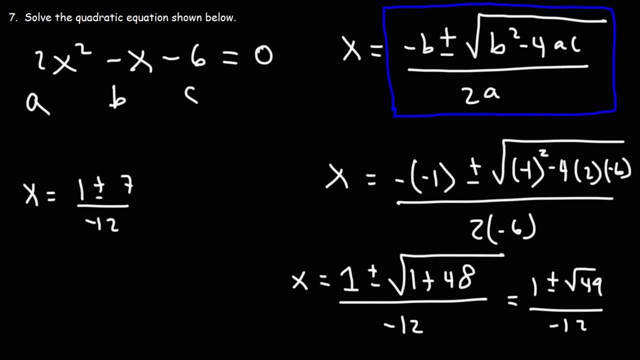 So now we get two possible answers. The first one is going to be 1 plus 7,, which is 8, divided by negative 12.. The other one is 1 minus 7,, which is negative 6, divided by negative 12.. 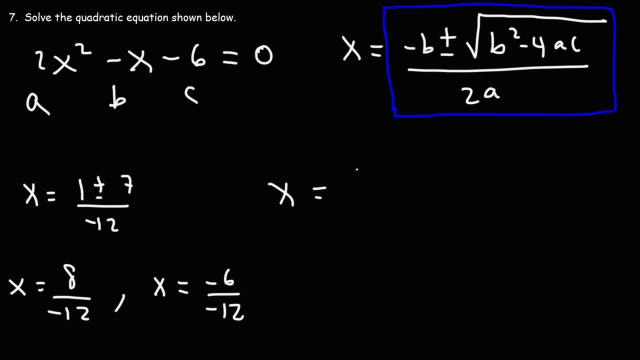 8 over negative 12.. We can write that as negative: 8 over 12.. 8 is 4 times 2.. 12 is 4 times 3.. The 4s will cancel. It doesn't matter if the negative is on top or on the bottom. 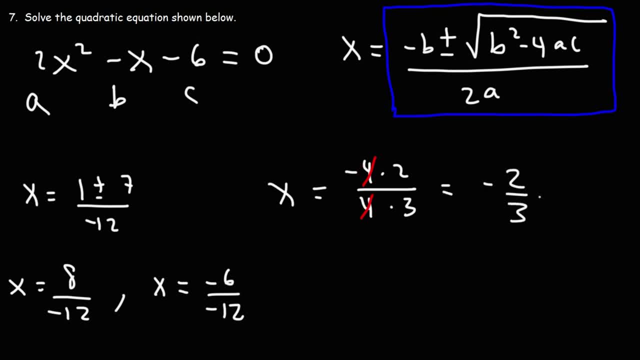 The whole number will still be negative. So we get negative 2 over 3. as one of the answers For the other one, we can write negative 6 as negative 6 times 1, and negative 12 as negative 6 times 2.. 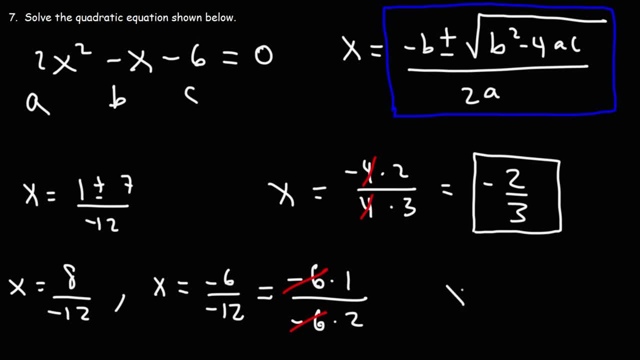 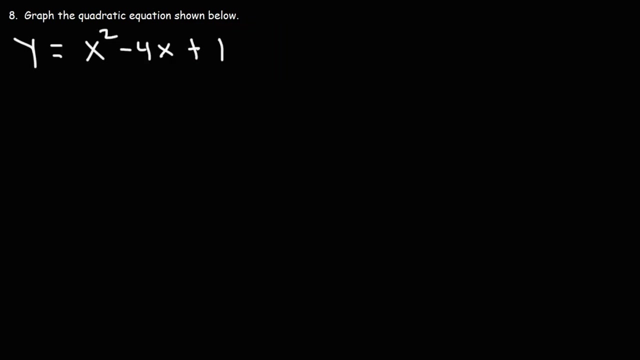 We could cancel negative 6, and that leaves us with the other answer, 1 over 2.. So those are the two answers in this problem. So that's how you could solve this quadratic equation using the quadratic formula. The next type of problem that 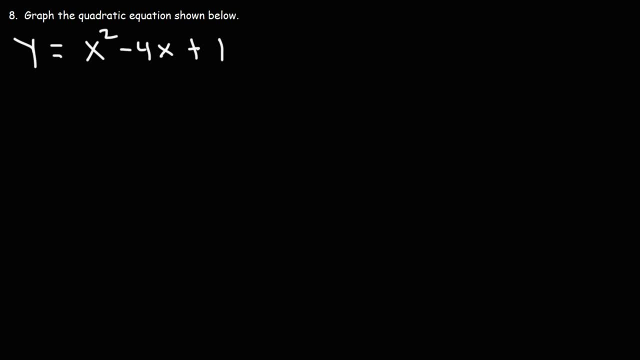 we're most likely to encounter has to do with graphing quadratic equations. Now, what I like to do is I like to find the axis of symmetry first. By the way, the generic graph is going to be the axis of this equation. Okay, 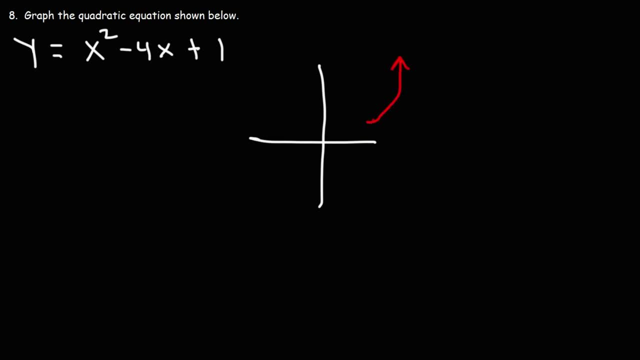 it's gonna look something like this: It's usually a parabola that opens upward or downward. If you have a graph that's positive x squared, it's gonna open upward. If it's negative x squared, it's going to open in a downward direction. 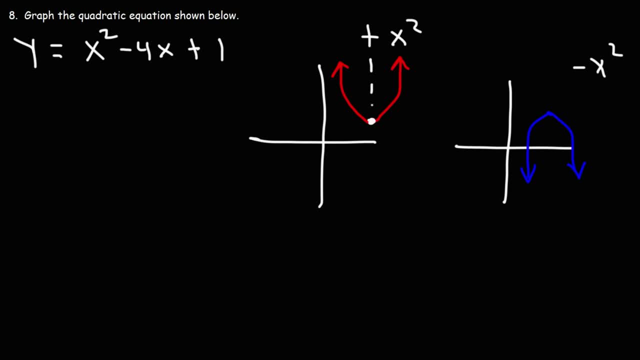 This point here is known as the vertex, And the vertical line that passes through the vertex is known as the axis of symmetry, And it's equal to some number, h. The coordinates of the vertex are h, comma, k. What I'd like to do is I'd like to find: 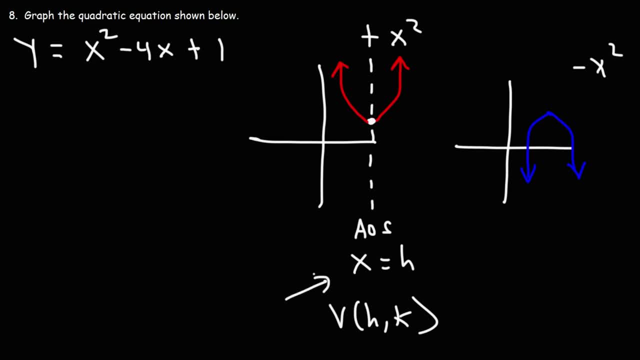 the x coordinate of the vertex and then make a data table around that point, because that's like the center of the graph. To find the x coordinate of the vertex you could use this formula: It's negative b over two a. So keep in mind a is the number in front of x squared. 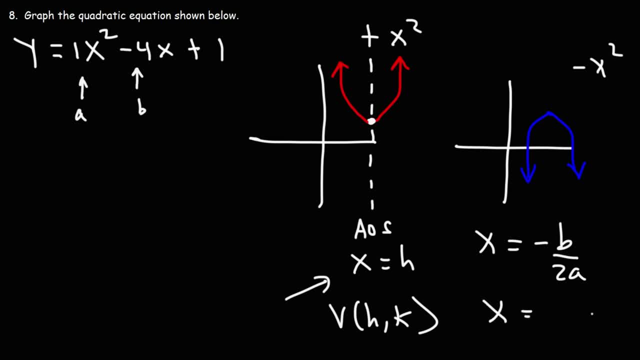 b is the number in front of x, So b is negative four. a in this example is one, So negative negative four over two, that's gonna equal positive two. So that is the x coordinate of the vertex. So now let's make a table. 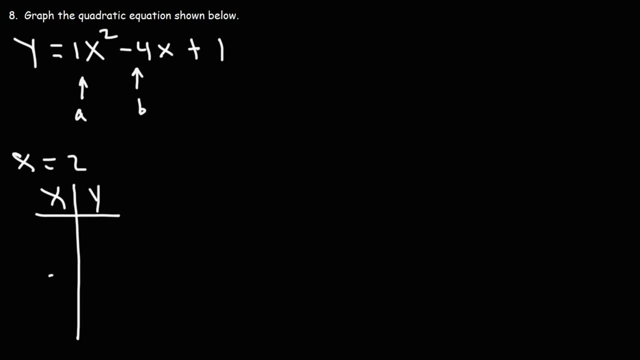 As I brought up in the previous video, I'm gonna use the same formula to find the x coordinate or the y coordinate of the vertex. So I'm just gonna use the x coordinate of the vertex and then double check that. If you see, here I have two points on the right of two. 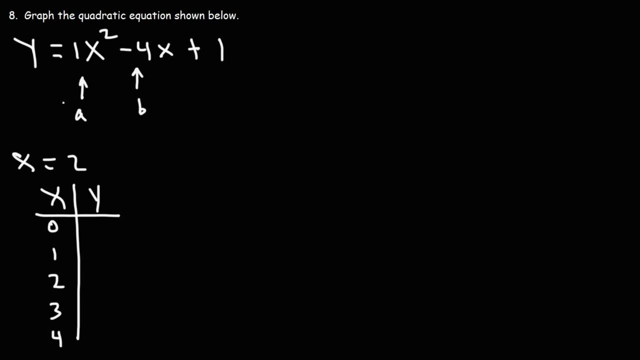 and two points on the left of two. So two is gonna be my center point. I'm gonna pick two points to the right of two and two values to the left of two. So the points I'm gonna choose are zero, one, two, three and four. 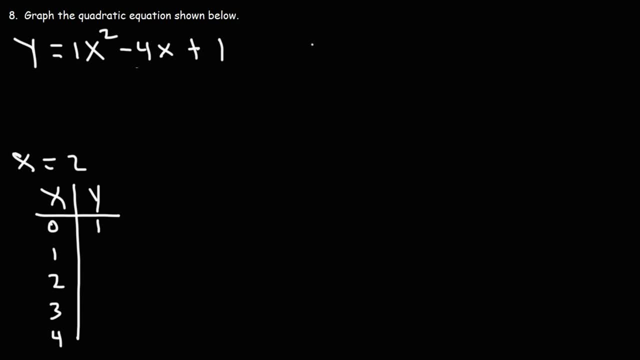 in 1 into this equation, this is going to equal negative 2.. If we plug in 2,, this is going to equal negative 3.. Now this is the axis of symmetry at x equals 2.. This is the vertex: 2, negative 3.. So the points to the left of this is going to be the same as the. 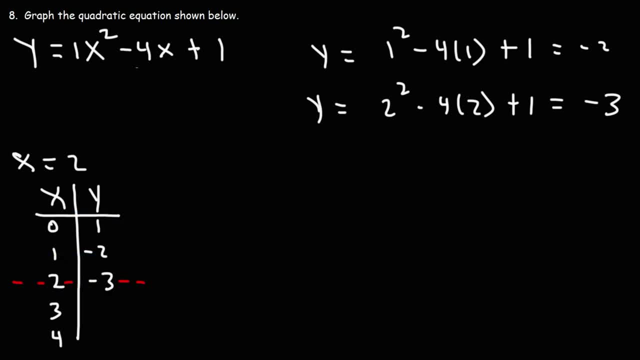 points to the right of it. This is why I like to center the table at the vertex. So since we have the point 1, negative 2, we're also going to have the point 3, negative 2.. Since we have the point 0, 1, we're going to have the point 4, comma 1.. And you could try it. 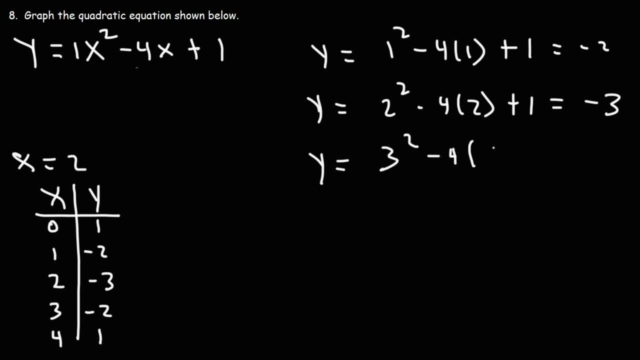 out. If you plug in 3,, you're going to get negative 2.. This is 9 minus 12 plus 1.. 9 minus 12 is negative. 3 plus 1. We get negative 2.. If you were to plug in 4,, 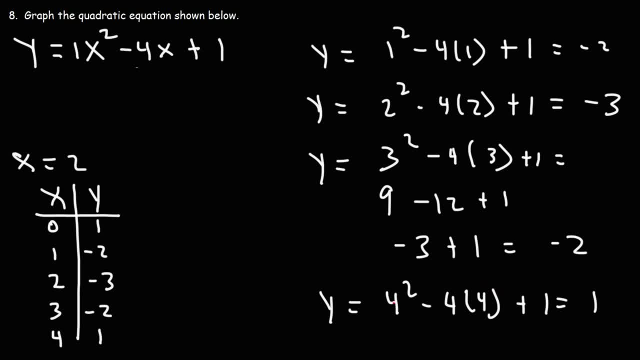 you're going to get positive 1.. 4 squared is 16.. 4 times 4 is 16.. Those two numbers will cancel giving us 1.. Now let's go ahead and graph this thing. So the majority of the 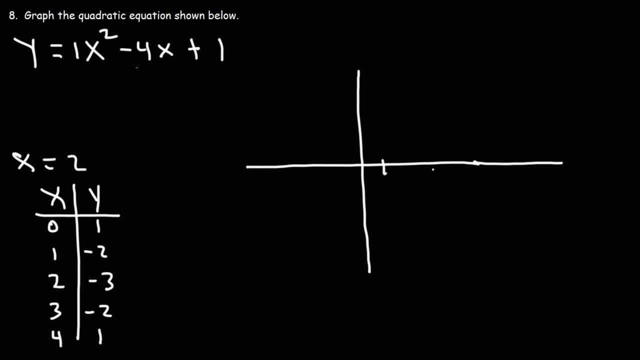 graph will be on the right side. So let's start with the vertex, which is that 2, negative 3.. So that's over here. Next we have the point 3, negative 2.. So x is 3, y is negative 2.. And then we have the point. 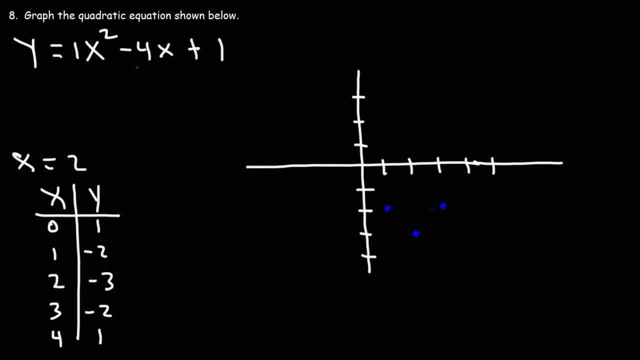 1, negative 2,, which is here, And then we have the point 0, 1.. So that's the y-intercept, That's where it touches the y-axis, And then we have the point 4, 1,, which is here, And you can see the symmetry between. 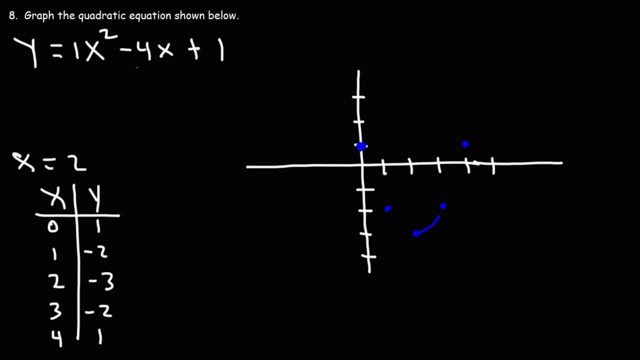 the points. That's why I've chosen them that way. So we're going to have a parabola that opens upward, since we have a positive x squared graph. So that's a rough sketch of this quadratic function. Another common topic that you're going to see in algebra has to do with 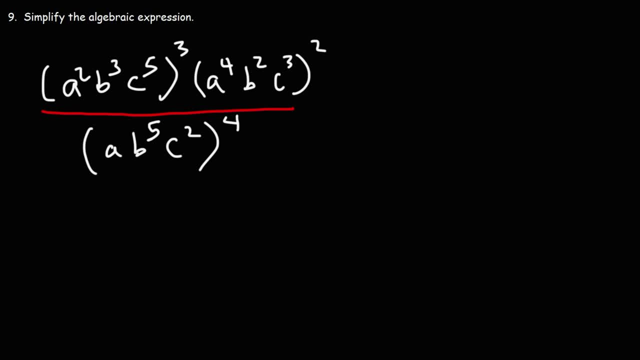 probability Properties of exponents. So here are some rules that you need to know. When you multiply by two common variables, you need to add the exponents 2 plus 3 is 5.. When you're dividing, you need to subtract the exponents 6 minus 4 is 2.. When you raise one exponent to another, 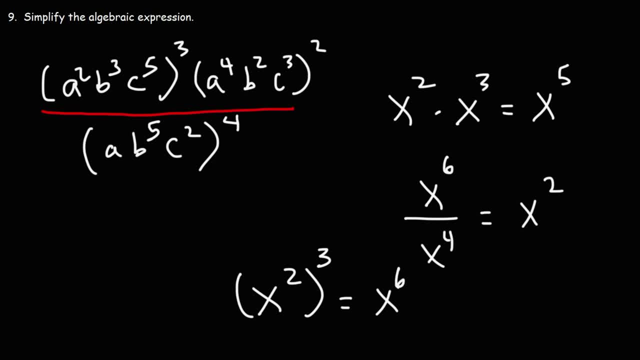 you need to multiply 2 times 3 is 6.. This is known as the product rule, the quotient rule And the power rule when dealing with exponents. So we're going to apply that here. Let's use the power rule first. So a squared raised to the third power When we raise one exponent. 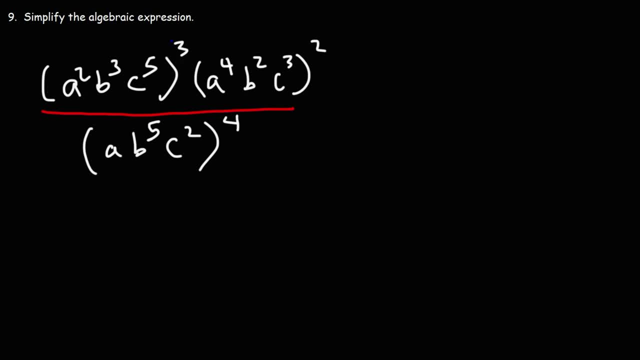 to another. we need to multiply, So we're going to distribute the 3.. 3 times 2 is 6.. 3 times 3 is 9.. 3 times 5 is 15.. Now this is multiplied to what we have here. 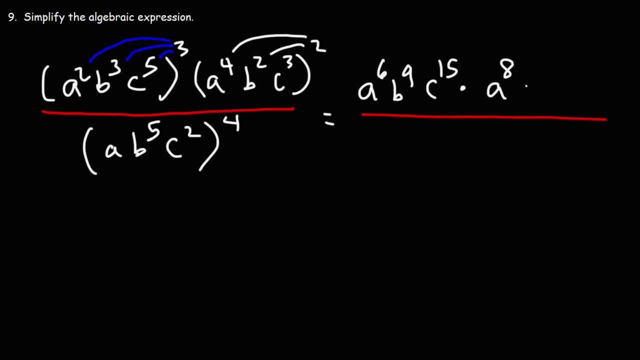 2 times 4 is 8.. 2 times 2 is 4.. And then 2 times 3 is 6.. Now we could do the same on the bottom. There's a 1 here, So we have 1 times 4.. 4 times 5.. 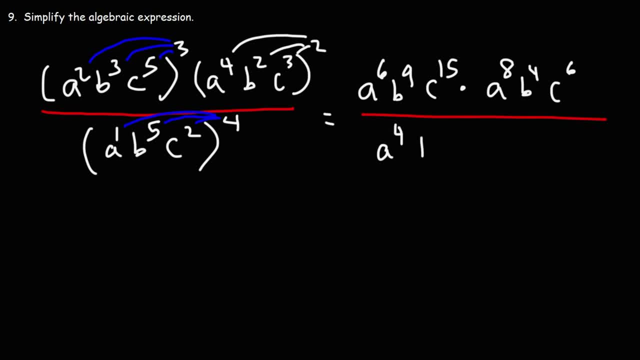 4 times 2.. So 1 times 4 is 4.. 4 times 5 is 20.. 2 times 4 is 8.. Now let's multiply. Whenever you multiply by two common variables, you need to add the exponents. 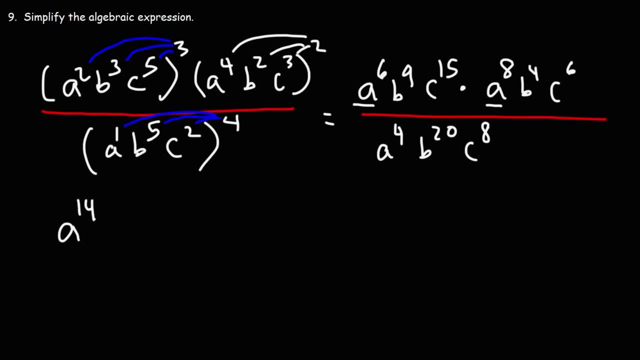 So 6 plus 8 is 14.. Here we have 9 plus 4.. That's going to be 13.. And then, if we multiply these two, we need to add 15 and 6, which will give us 21.. 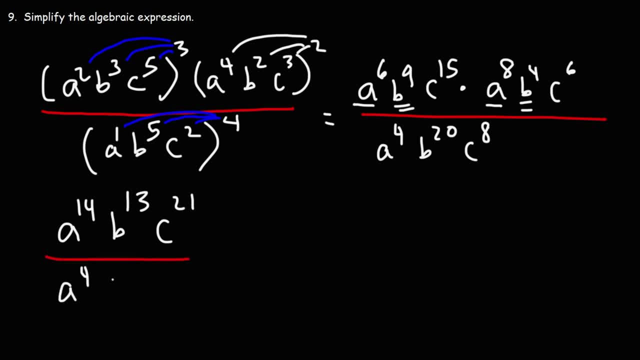 So now we need to divide. When you're dividing by two common variables, subtract. So 14 minus 4, that's going to be 10.. 13 minus 20 is negative, 7.. 21 minus 8 is 13.. 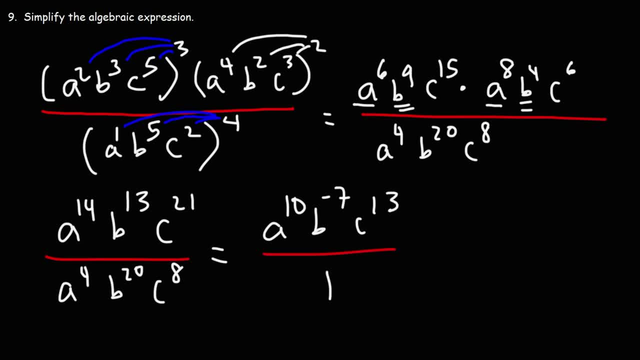 And this is going to be over. 1. Now notice that we have a negative exponent. In order to fix that, just move the exponents to the right. Just move the exponents to the left. Just move the variable to the other side. 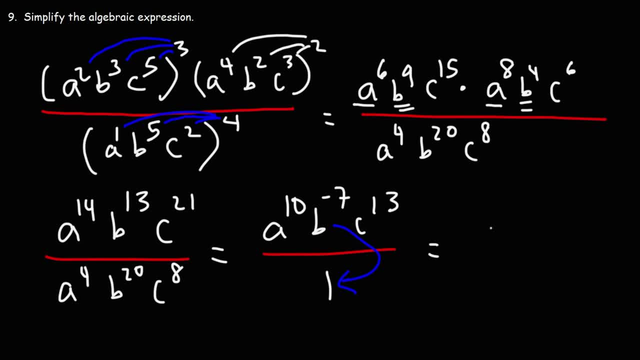 The negative exponent will become positive. So the final answer is a to the 10 times c to the 13, divided by b to the positive 7.. So that's how you can use the properties of exponents to simplify an algebraic expression like this one. 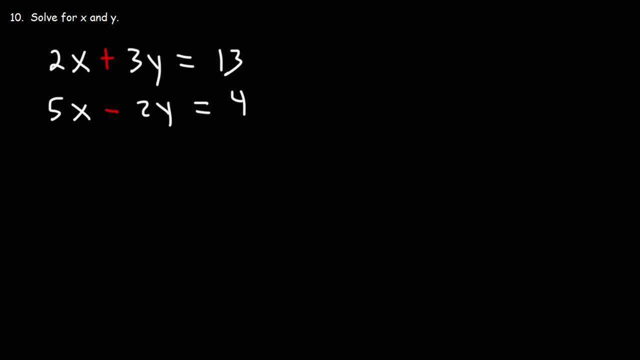 The next common type of problem is solving a system of equations. Here we have a system of two linear equations. Sometimes you may need to solve a system of three linear equations, in which you'll have three variables: x, y and z. Other times you may need to solve a system of two quadratic equations. 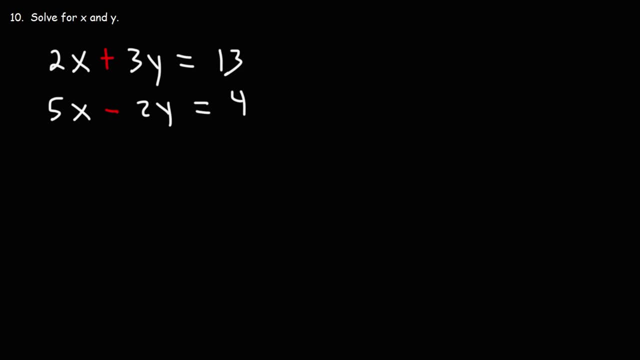 I've seen those, But let's focus on this problem. There's two methods. we could use The substitution method or the elimination method. I'm going to use the elimination method for this example And I'm going to focus on canceling the y variable. 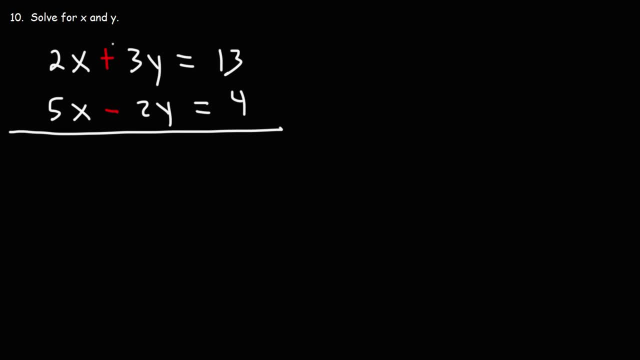 Right now. if we were to add the two equations, the y values won't cancel because they're not the same. So I'm going to multiply the two equations in such a way that the y values will cancel. The least common multiple of 2 and 3 is 6.. 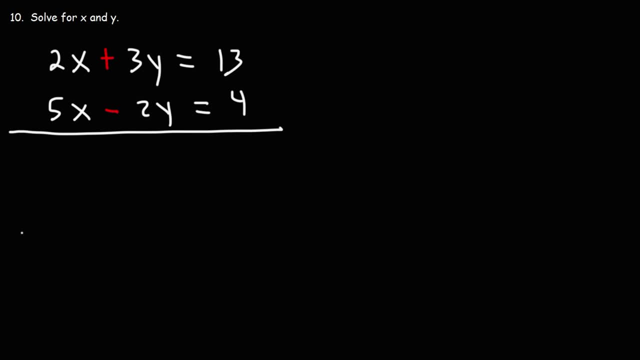 So I need to make this positive 6y and negative 6y. So I'm going to multiply the first equation by 2 and the second one by 3.. So we're going to have 4x plus 6y equal 26.. 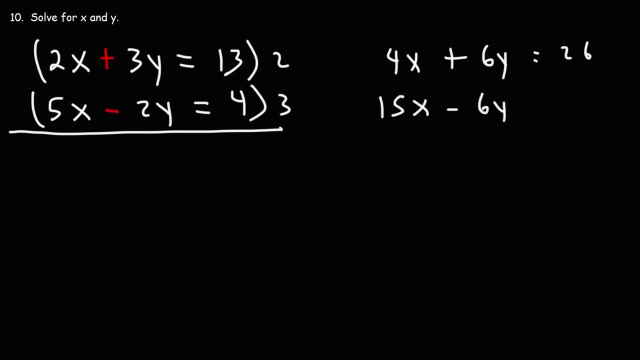 And for the other one we're going to have: 15x minus 6y equal 12.. These two will cancel, And so we're going to have: 19x is equal to 26 plus 12 is 38. If we divide both sides by 19,. 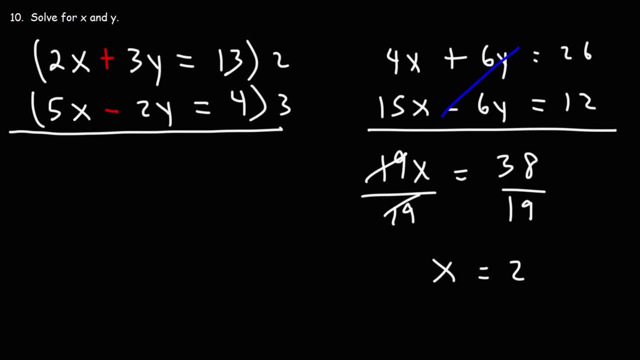 38 divided by 19 is 2.. So we get: x is equal to 2.. Now, once you have x, you can calculate y. Let's plug it into the first equation before you multiply it by 2.. That is this one here. 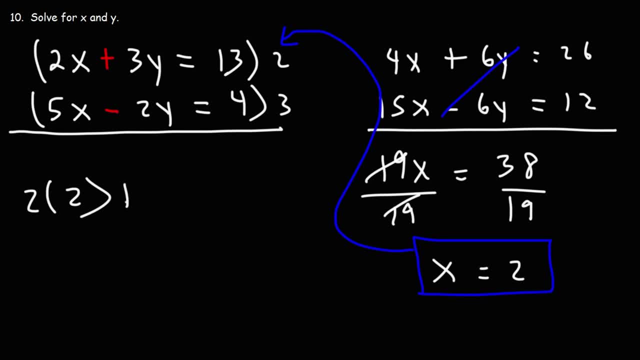 So I'm going to replace x with 2 and I'm going to solve for y. 2 times 2 is 4.. Subtracting both sides by 4, we get 3y. if we bring this down is equal to 13 minus 4,. 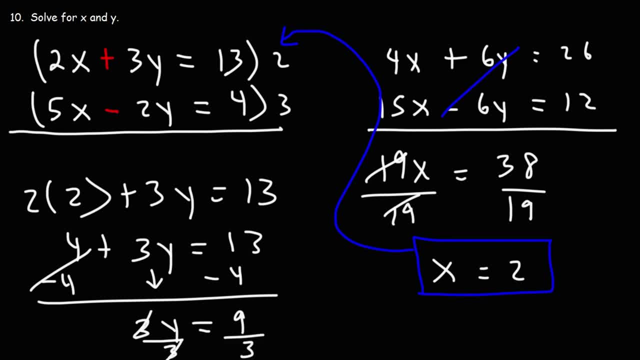 which is 9.. Dividing both sides by 3, 9 divided by 3, is 3.. So the two answers are: or the answer is x is 2 and y is equal to 3.. So we can write the answer as an ordered pair. 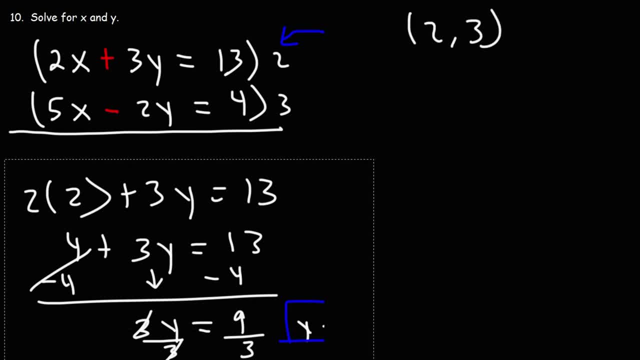 We can leave it as 2 comma 3.. Now, if you want to check your answer, you can plug this in back into the original equation. So if we plug it into the first equation, we can see if the left side is equal to the right side. 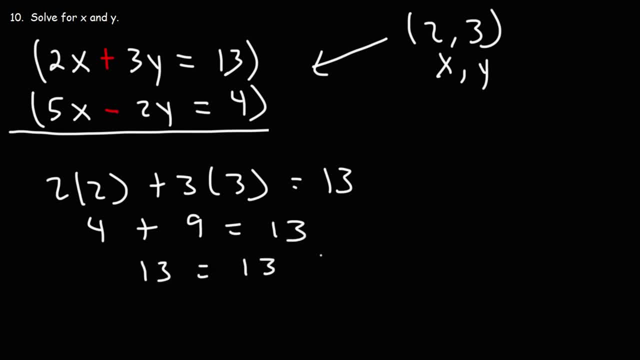 4 plus 9 is indeed 13.. So this works. If we plug it into the second equation, we'll have 5 times 2 minus 2 times 3.. Let's see if that equals 4.. 5 times 2 is 10.. 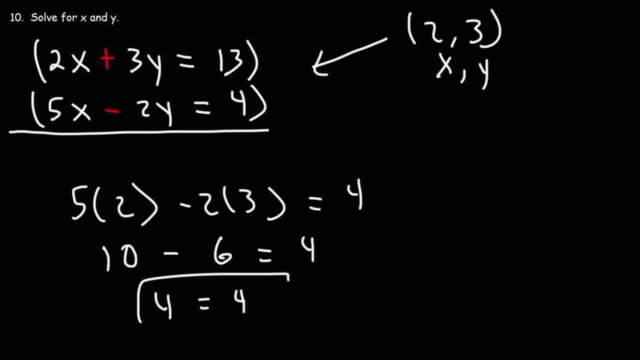 2 times 3 is 6.. 10 minus 6 is 4.. So this answer is indeed correct. So those are 10 common types of problems that you'll see in a typical algebra course in high school or in college. Linear equations. 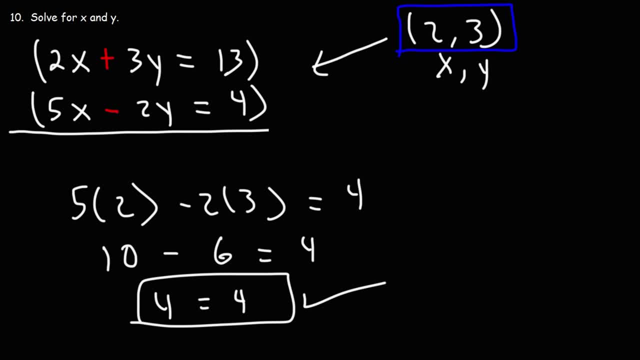 solving them, graphing them, calculating the slope, writing linear equations. and then you have quadratic equations: factoring it, solving it, graphing it. system of equations simplifying algebraic expressions, property of exponents, inequalities, just to name a few. 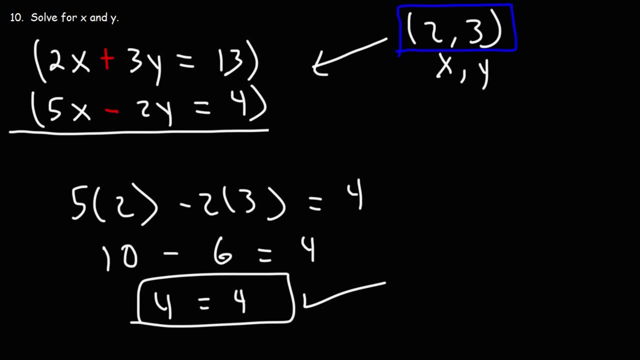 Now there are other topics too that you might see, like logarithms, radical equations, rational equations and other stuff like that.